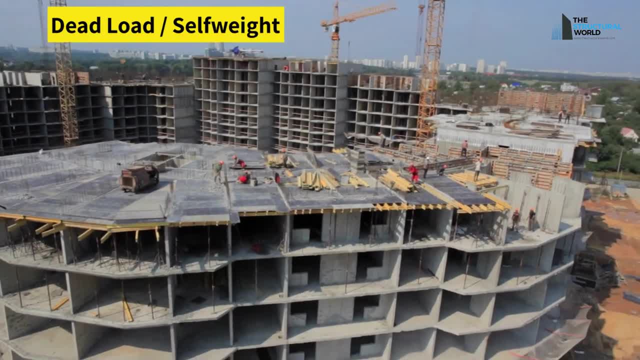 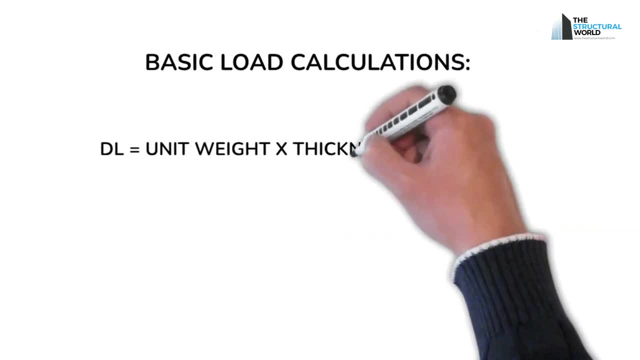 We will start our calculation from there. Dead load: Dead load is the self-weight of the structure. To calculate dead load, the density, or unit weight, of the structure should be multiplied by the thickness. That will give us the weight of the structure per given area. 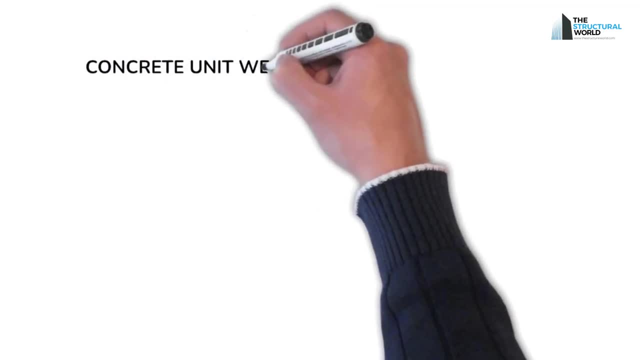 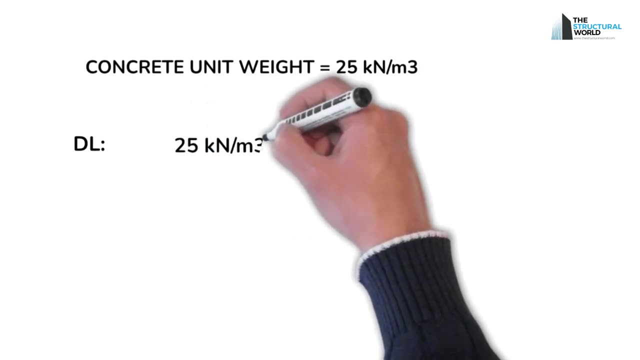 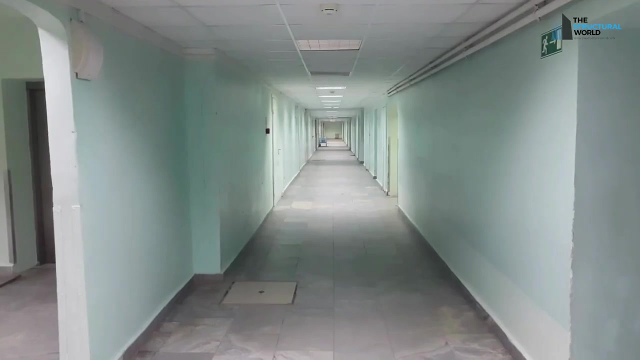 For a concrete slab of 0.25 meters thick, for example, that will give us the following: Considering unit weight of concrete to be 25 kilonewtons per cubic meter, 25 kilonewtons per cubic meter multiplied by 0.25 meters equals 6.25 kilonewtons per square meter. 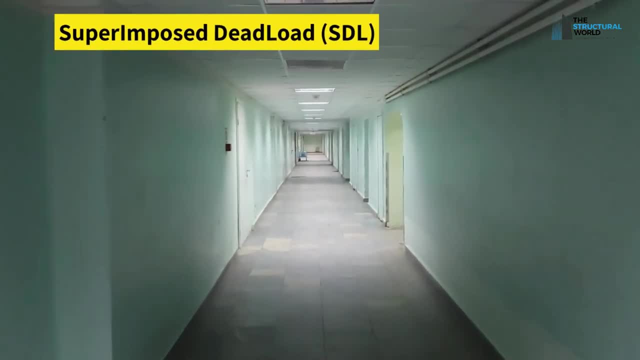 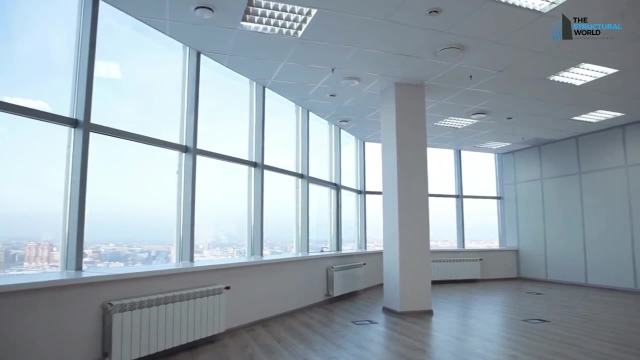 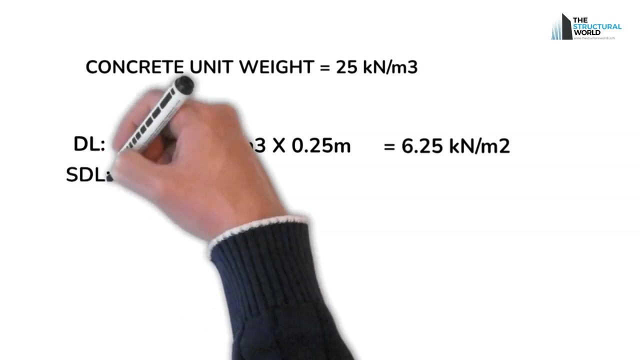 Superimposed dead load. Superimposed dead loads include the partition or interior walls, floor screed, floor finish, ceiling loads, façade and internal cladding and MEP pipes and fixtures. To calculate, let us assume that a slab is carrying a total of 6 kilonewtons per square meter. 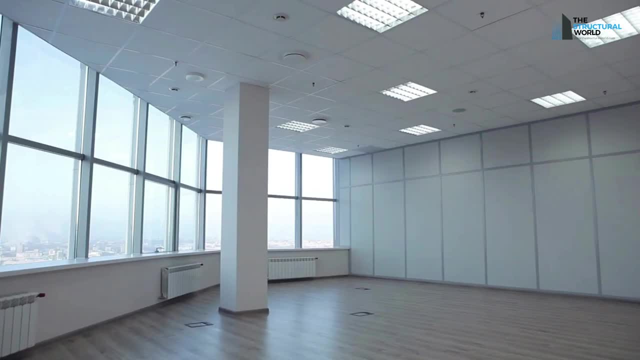 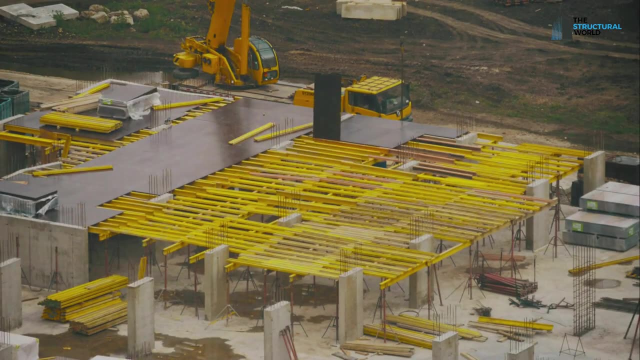 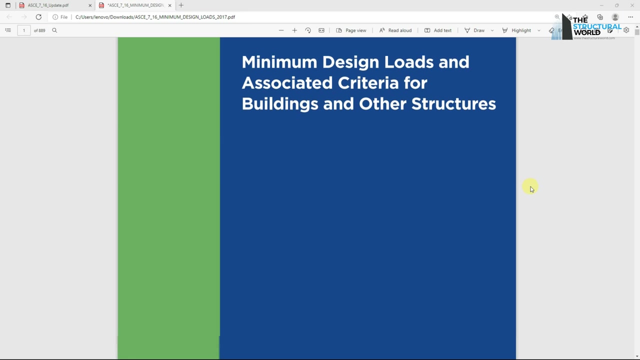 Note that the same principle as calculating dead loads can also be adopted in determining the weight of the superimposed dead load making up the construction with the given density or unit weight of the material. These densities or unit weight of materials can be sourced from the relevant codes and standards, material data sheets or obtained via laboratory testing. 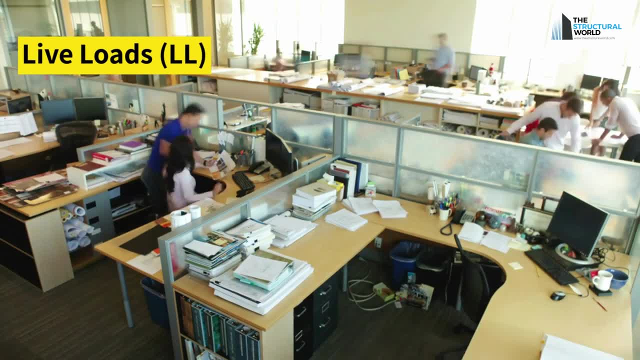 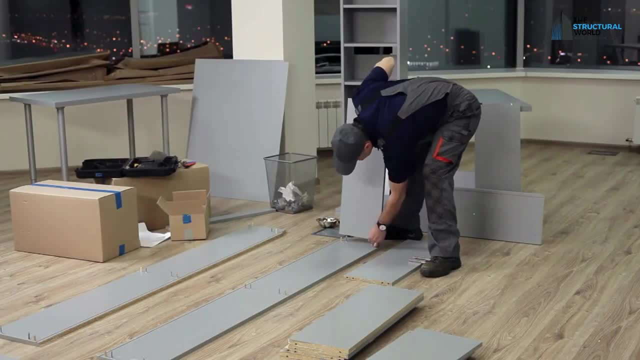 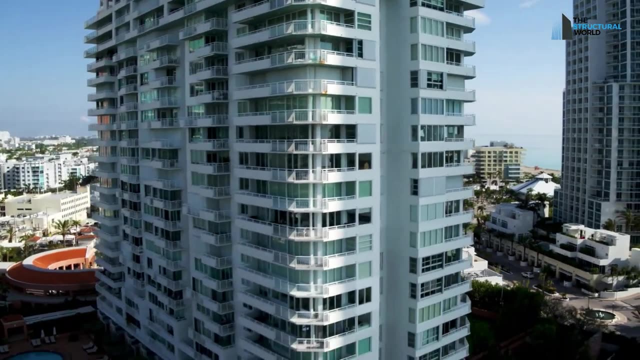 Live load. Live loads are the movable or moving loads that the structure can carry. It can include the movable equipment, movable partitions, furniture and other people occupying the structure. Live load assumptions depend on the usage of the building or type of occupancy. It has obviously bigger live loads in an assembly or gym areas. 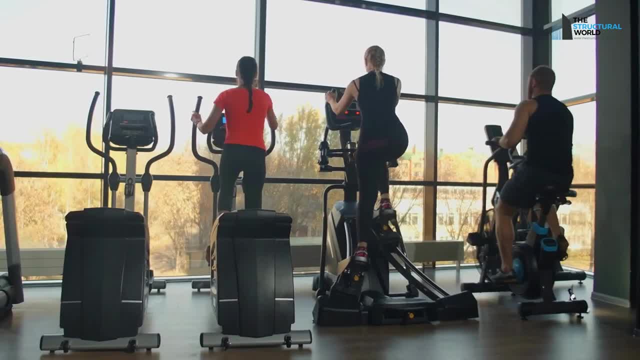 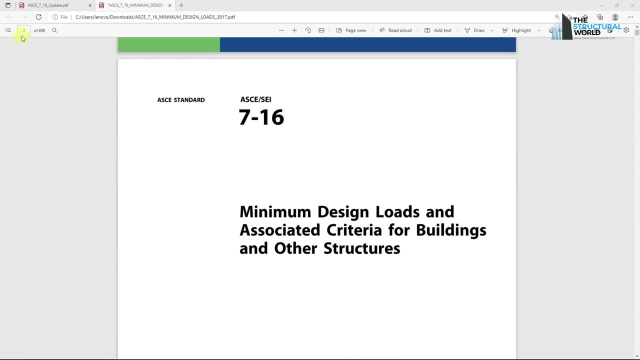 as compared to the residential areas. The minimum live load requirement is given in the codes and standard that we are using. Referring to ASCE 7-16, for example, table 4.3-1 will give you all the recommended live loads of the structure being designed. 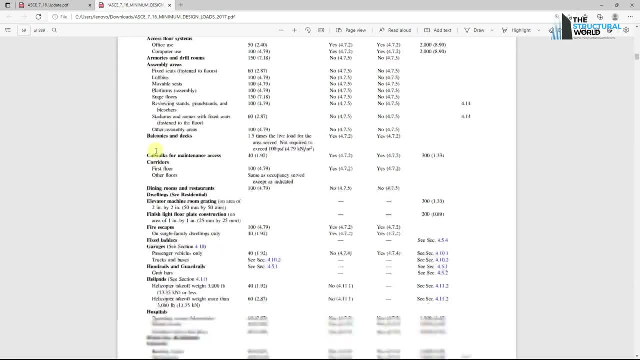 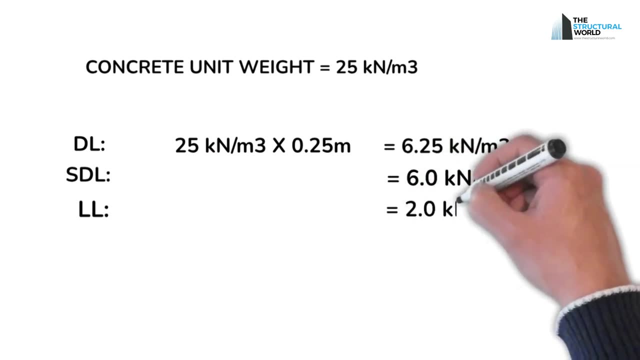 Let's take the live load to the 2 kilonewton per square meter, So our live or imposed loads on a residential concrete structure can be summed up to dead load or self-weight- 6.25 kilonewton per square meter. 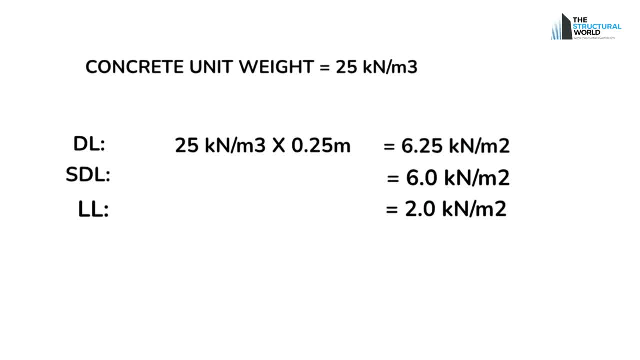 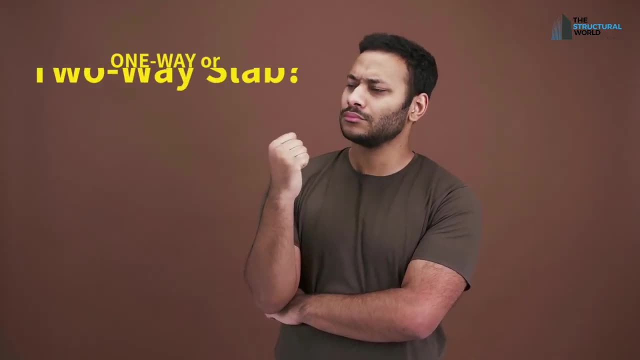 Superimposed load 6 kilonewton per square meter And live load: 2 kilonewton per square meter, How the basic load is being distributed in the structure. Before we proceed, you have to differentiate whether our slab is a one-way or two-way slab. 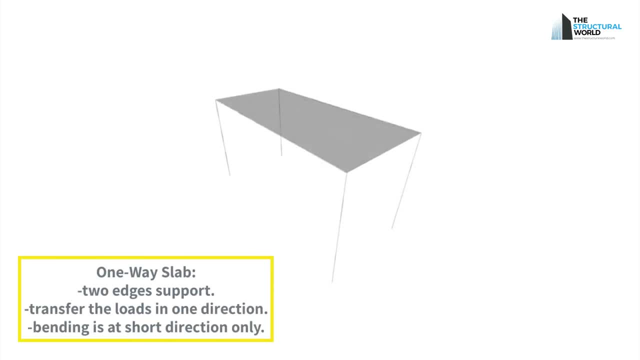 One-way slab transfers the imposed loads in one direction only or in two edges to the perpendicular beam or walls. This tends to bend the slab in a short direction only. The two-way slab has four edges support. It is supported by beams or walls on all four sides. 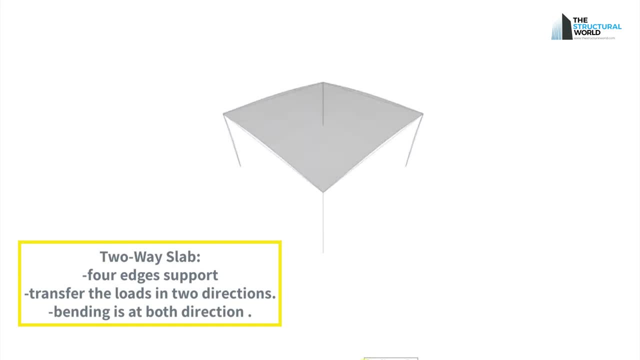 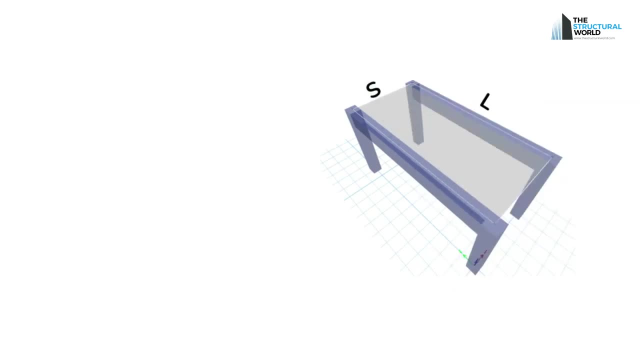 in which the bending occurs in two directions of the slab. To verify using calculations, we can see the following formula For a one-way slab: we can consider a one-way slab if the ratio of the longer to the shorter span of the slab is greater than 2.. 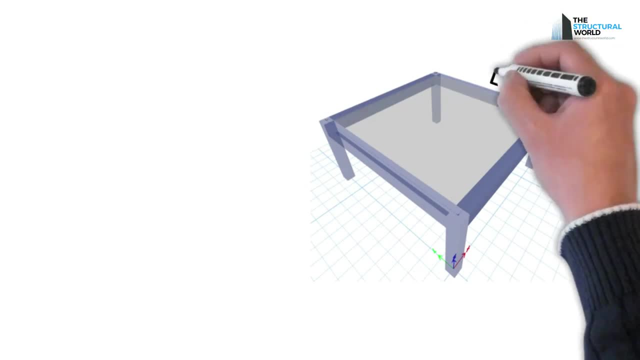 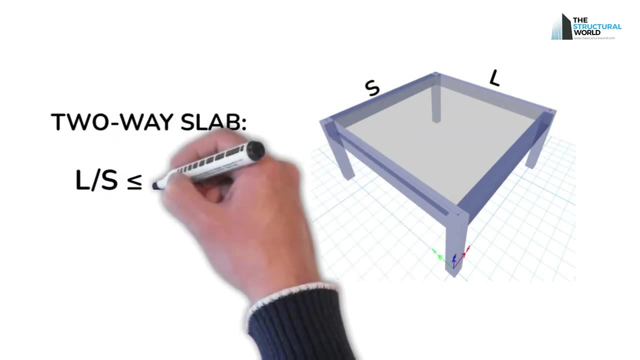 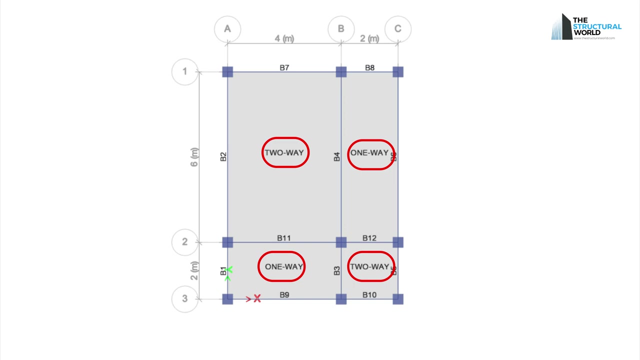 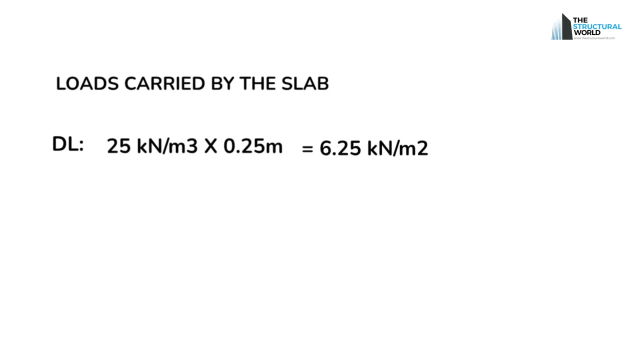 And for two-way slabs, the ratio of longer to the shorter span of the slab is less than or equal to 2.. Applying the formula for slab classification, let's now look at this slab framing layout as an example To distribute the loads. let us consider the result of the loads that we previously calculated. 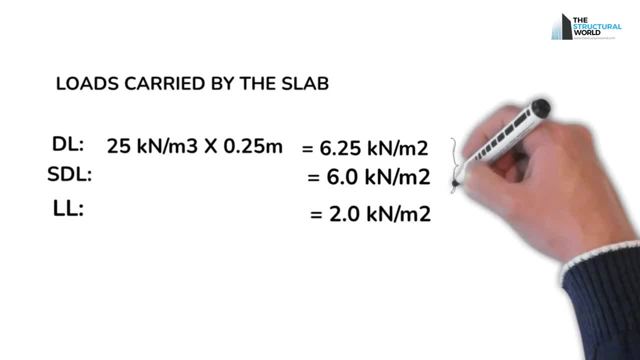 Total dead loads: 12.25 kilonewtons per square meter. Total live load would be equal to 2 kilonewtons per square meter. The dead load, superimposed dead load and live load that we consider will be carried by the slab. 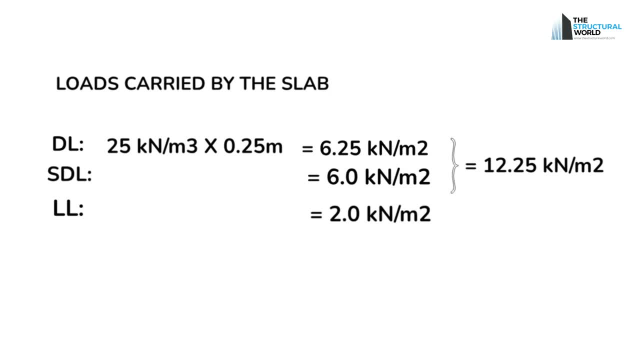 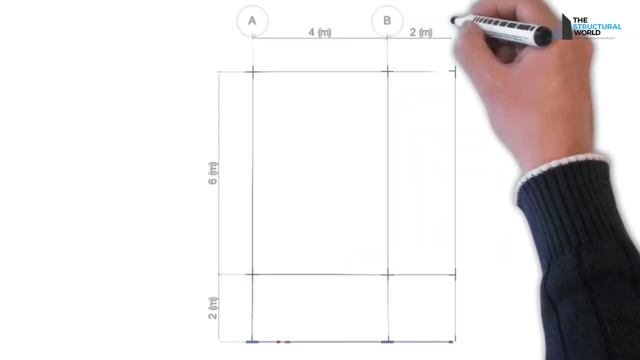 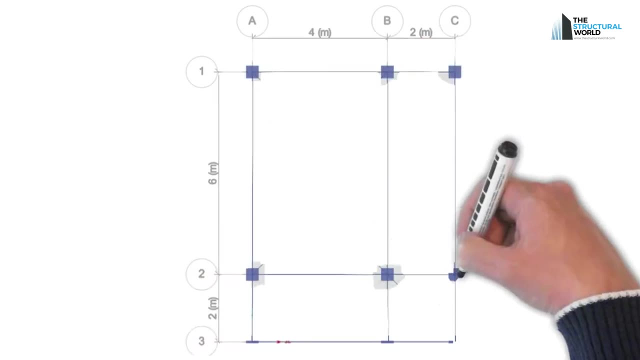 It will then be distributed to the perimeter beam supporting it. To distribute it on the perimeter beams, let's take a look at this figure. To distribute the load on a two-way slab, simply draw an isosceles triangle in its short direction. 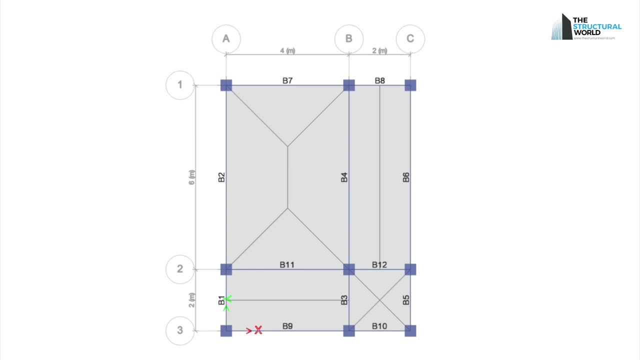 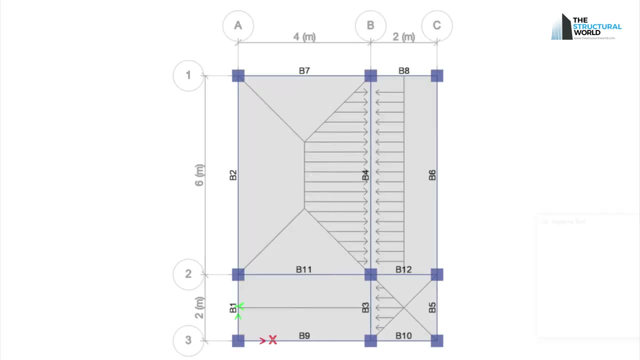 and a trapezoid in its long direction. as shown, A one-way slab simply cuts the slab into two along its length. For the beam to carry the slab, calculate the areas adjacent to it. Let's calculate the loads on beams B3 and B4, respectively as an example. 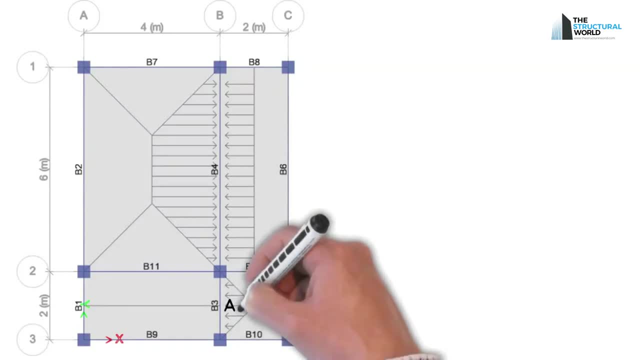 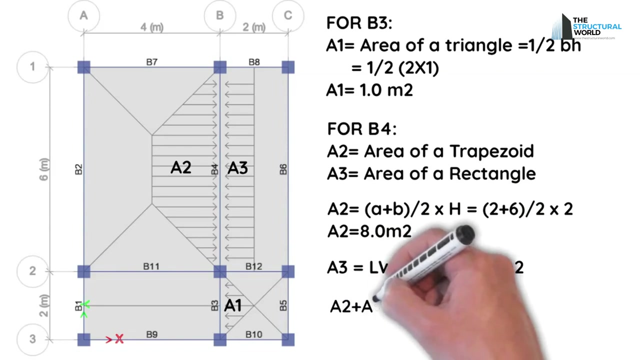 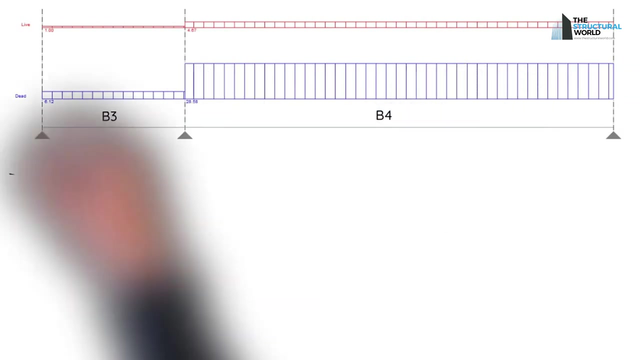 Area of triangle at B3 equals 1 square meter. Areas adjacent to B3 equal area of trapezoid plus area of rectangle equals 14 square meters To distribute it along the beam. multiply these areas with the dead load, superimposed dead load and live load to get the actual load distribution in kilonewton.